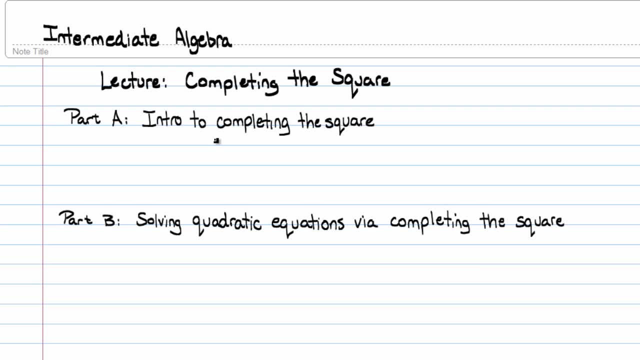 We're going to talk a little bit about what completing the square really means geometrically. As most of my lectures, as I try to do in most of my lectures, we'll try to have a very common sense approach to this idea of completing the square and what we can use it for. 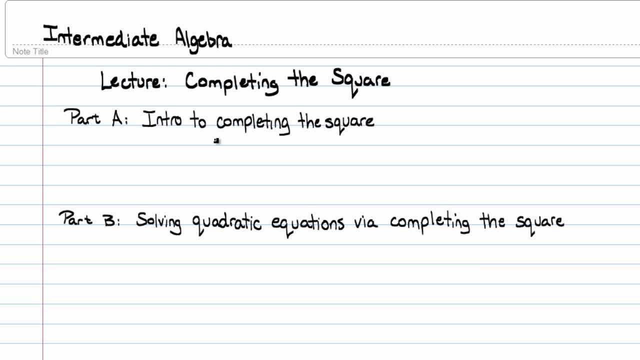 Specifically, we're going to talk about using it for solving quadratic equations, and that's what we're going to do in the second part of this video lecture, But really it would be best for you to watch the first part so that you can really understand the idea behind why we complete the square. 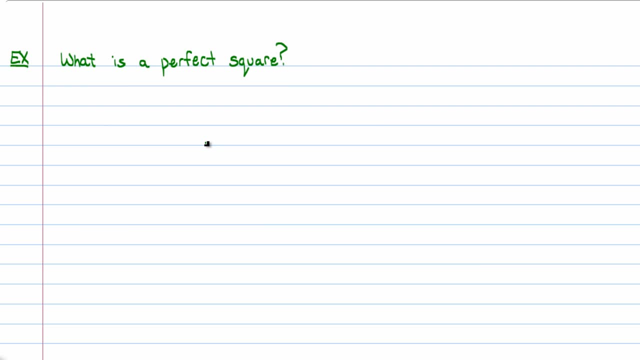 So here we go, Let's talk about that. We'll start the whole thing with a discussion on what is a perfect square. In mathematics, a perfect square takes on a different style of definition, but a lot of people if you just walk around and say what's a perfect square? 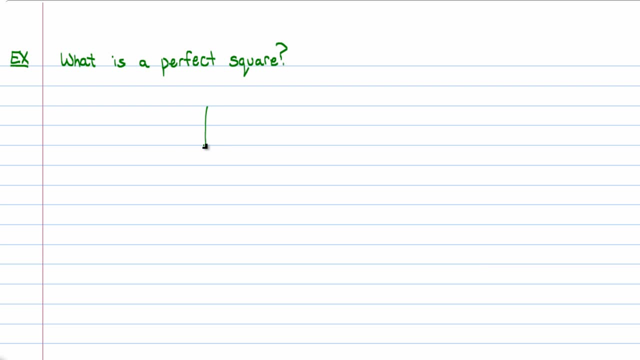 people usually think geometrically as it being a square where all sides are of equal length, which is the definition of a square, but they'll call that a perfect square because they think that a lot of people think that if let's say it's somewhat elongated. 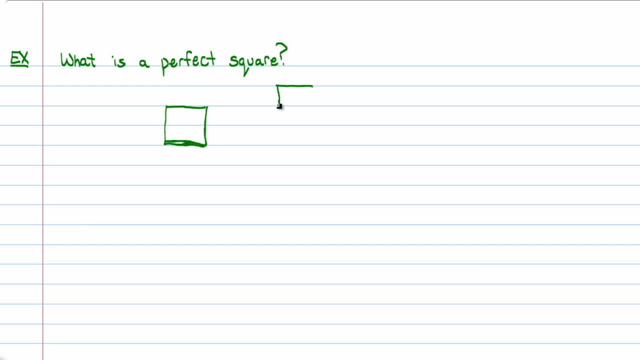 so, in other words, if something like this, that this is not a perfect square, That is actually not even a square, that's just a rectangle, But a square, is this object right here And, like I said, a lot of people consider that to be perfect as far as squares go. 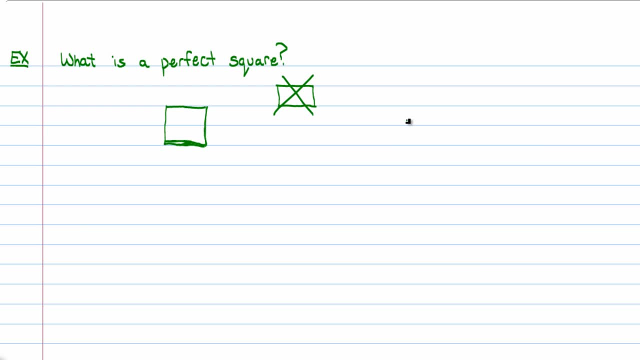 I don't know why. In mathematics, a perfect square is a number that is well the product of two numbers that are the same. So let me write that down: A number b is a perfect square if there's something like this. 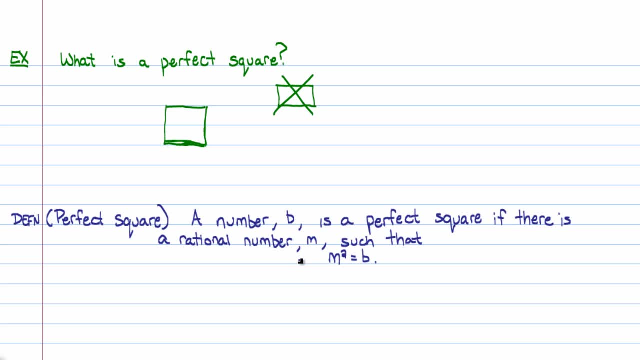 Some rational number, some number that we know, that's a nice number. a rational number, m, such that m squared is equal to b. We have some pretty quick examples. For example, 9 is a perfect square because 9 is equal to some number squared. 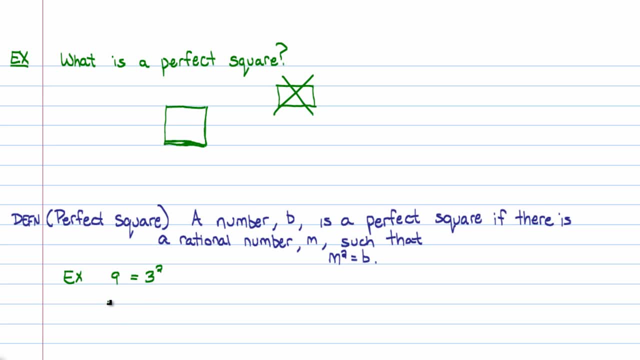 specifically 3 squared. You know you go down that list. you could say 16 is a perfect square because, well, 16 can be written as a rational number squared. But even let's say 9, 49ths is a perfect square because it can be written as a rational number. 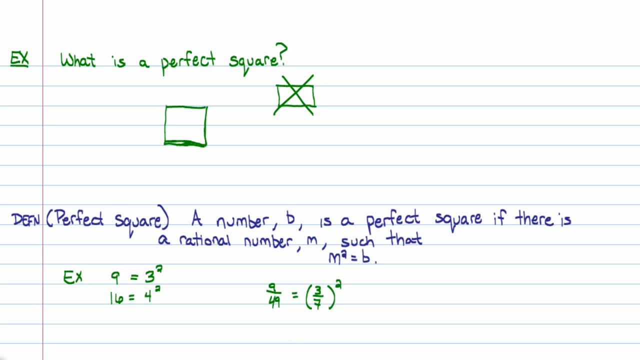 a fraction squared, a 3 7ths squared. But remember, a rational number is a ratio of integers, so something that's not a perfect square is like the number 7. Even though 7 actually, if some people might know. 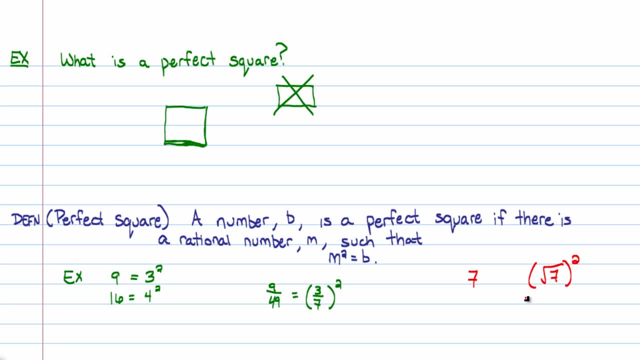 7 is actually equal to the square root of 7 being squared. The square root of 7 is not a rational number, so we cannot include that in the set of our perfect squares. We can't include 7 in the set of perfect squares. 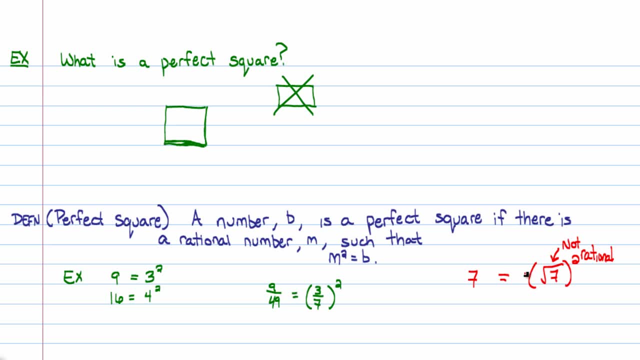 because it's not a square of a very perfect number. So just remember that To be a perfect square, your number that you're looking at has to be the square of some nice number, some either integer or fraction. The question comes up when you're talking about polynomials. 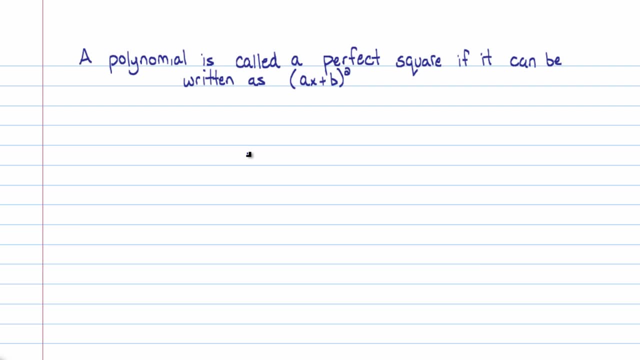 what does it mean to be a perfect square? So a polynomial is called a perfect square if it also can be written as a polynomial squared. A simple example of a perfect square polynomial is something like x squared plus 10 squared 10x plus 25.. 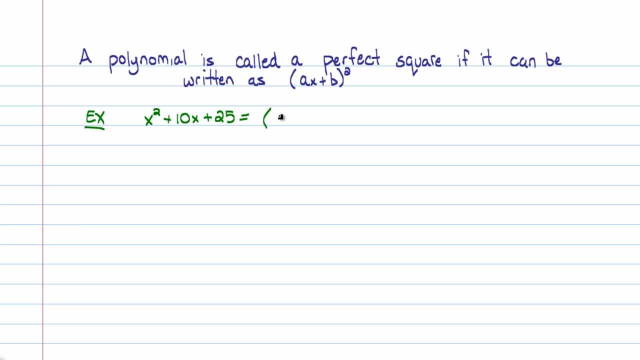 This is a perfect square polynomial because I can actually see that it's the same thing as x plus 5 times x plus 5, or in other words, x plus 5, quantity squared. The square notation means that this picture x plus 5. 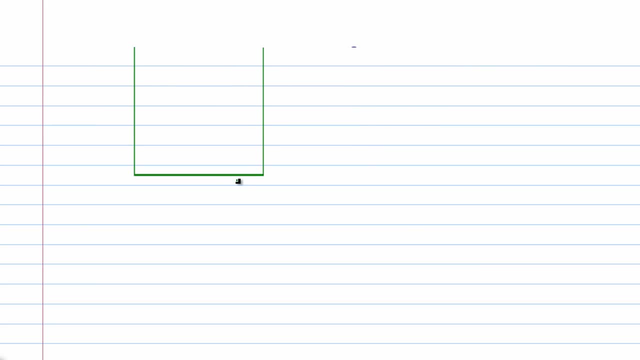 is just multiplying itself twice. But now let's get into the idea of how to make a polynomial a perfect square, And the way we're going to do this is to look at a nice square first. This is a square most people would agree. 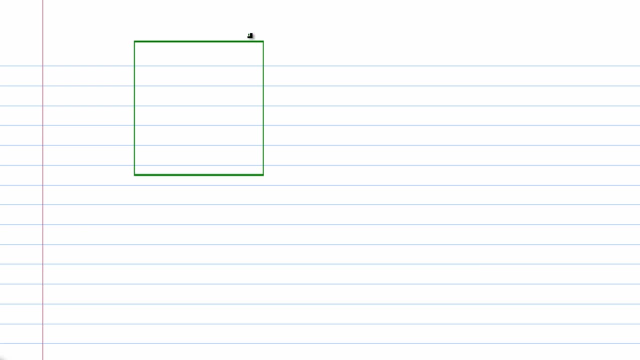 What I'm going to do is I'm going to pretend for a moment that this side length here is of side length. oh, let's say x. Well, if this is of side length x, then since it's a square, this vertical side length also should be of length x. 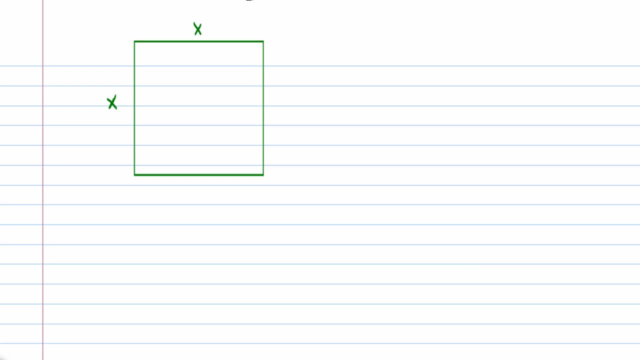 Now I'm just going to make up a number here, So what you're about to witness is not me knowing anything other than just making up some number for the width of this next little piece I'm putting on here. So let's just pretend that's a nice rectangle. 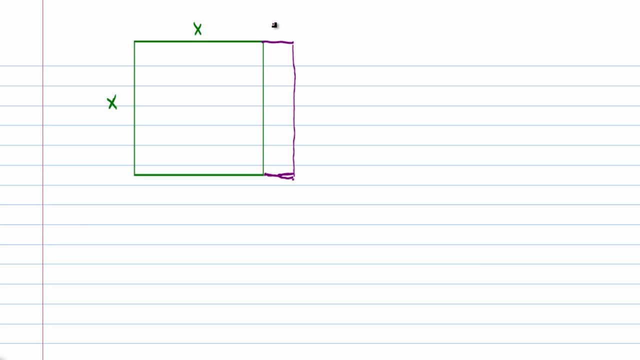 And let's pretend that I say, this little width here is a width of let's do 5, let's do 6, actually, because I already did a 5 a moment ago, So let's say that's of length, 6.. And at the same time, 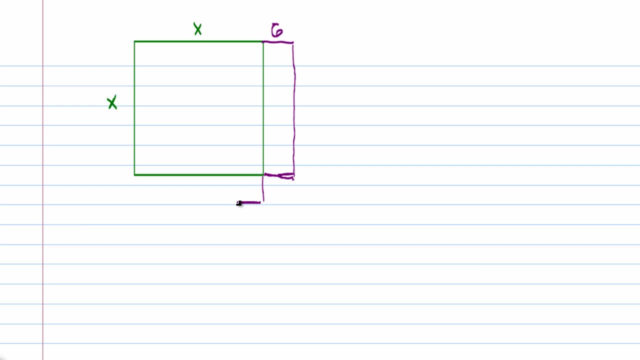 let's pretend that we have a block down here as well that we attach to this. So we have two of these purple blocks that we're attaching to this green square, And let's pretend this block has a height of 6.. First, I'm going to ask you. 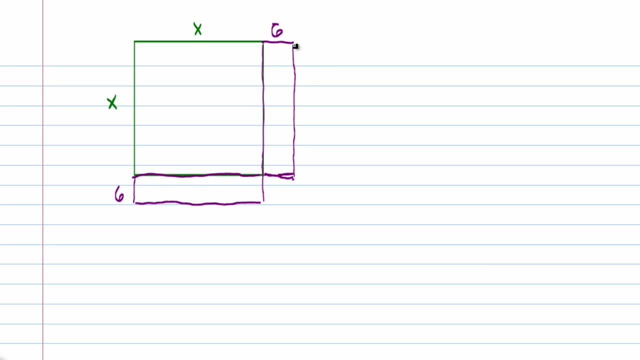 what is the height of this vertical rectangle? If you think about it, it has three sides. It's this high and it goes down this low. and we know the distance from here to here is just the same as the height of this square, which is x. 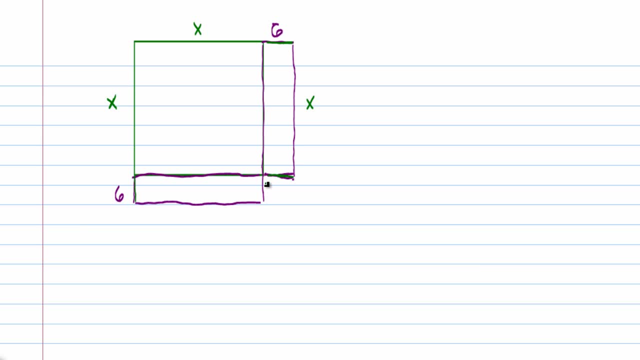 And if you look at the bottom rectangle, the width is the same as the width of the square, so that's a width of x as well, And what I'm going to ask is: what size little square do we need to put in here? 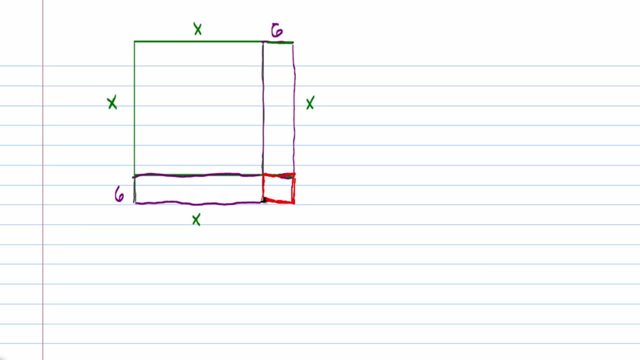 What size is that square? That will complete this square. So let me write that down. And when I say what size square would I add to this figure, I'm really asking: what is the size of this red square that I put in here? 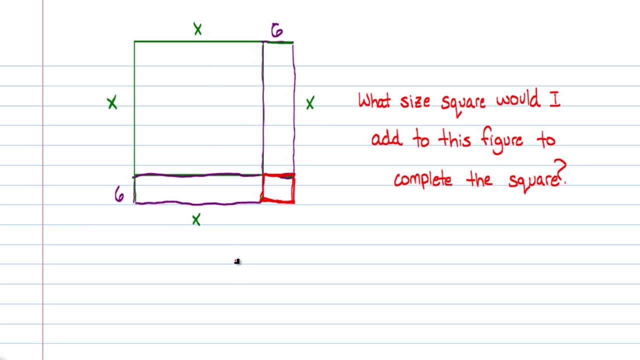 That would make this whole picture turn into a nice square. You see, this picture is actually a nice little square again. Well, if you look at that, it seems to me that the height of this little square is 6 and the width of this little square is also 6. 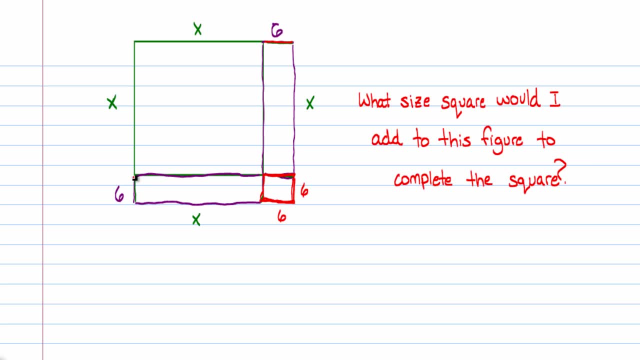 because I'm just matching it up to this width and this height, right? So let's stop for a moment and think about what just happened. Really nothing fascinating, it's just that somebody started with a square, an x by x square, and they put on two little blocks that were the same size. 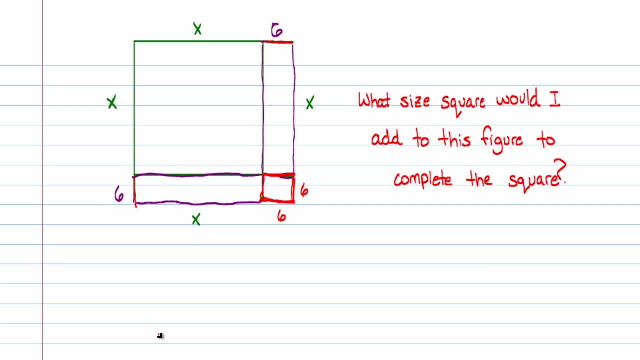 One was 6 by x, the other one was 6 by x And we said: what's that missing little piece? Well, it's easy to see: it's going to be a 6 by 6.. So that little area right in here. 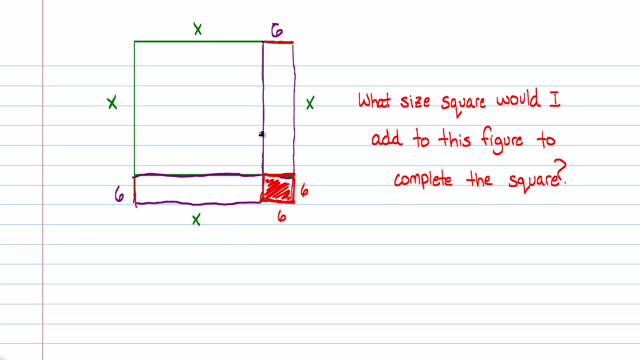 I'll shade in. right now it's just a little 6 by 6 area. But now let's talk about this and turn this into a polynomial. To turn it into a polynomial, I'm just going to ask: what is the area of this square right here? 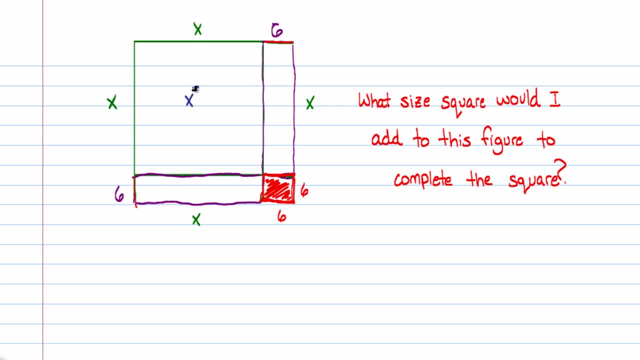 It's x by x, so the area here is x squared And the area of this tall rectangle is 6 by x, or in other words 6x, And the area of this long rectangle down here is 6 by x. 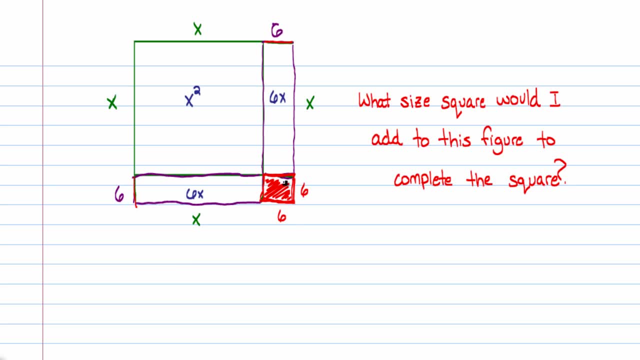 or in other words 6x, And the area of this red square that we had to add in here. that area is 6 by 6, or in other words 36.. So if we were given a polynomial x squared plus 6x plus 6x, 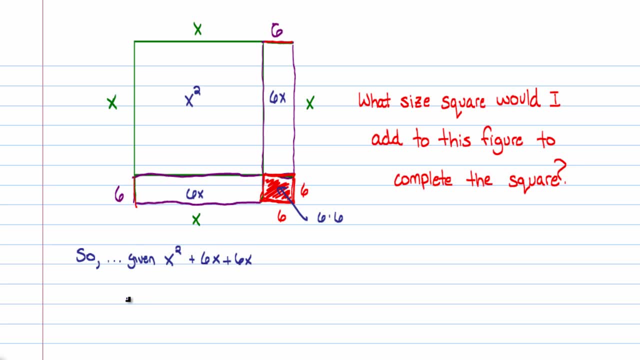 so if we're given that, so I'll write given in here, which, by the way, is actually equal to x squared plus 12x. If we're given that, to make this into a perfect square, we would just add 6 by 6,. 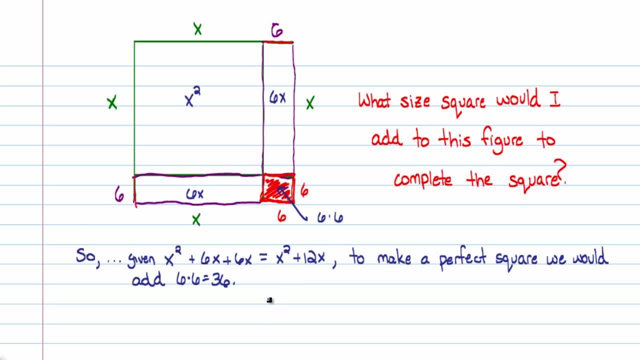 or in other words 36.. In other words, we would get something that looks like this: x squared plus 12x plus 36.. Now if you actually factor this polynomial, it does factor nicely to x plus 6 times x plus 6,. 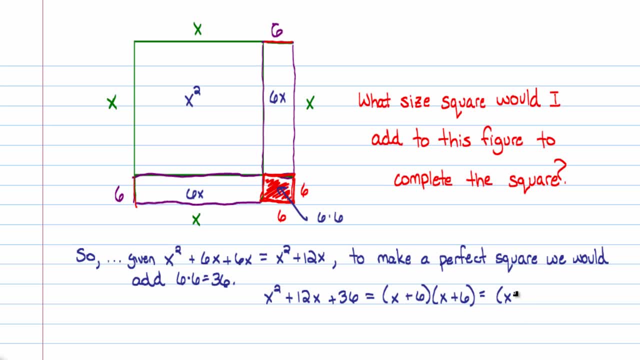 which is actually a perfect square, right? This is x plus 6, quantity squared. So, starting with this polynomial here, if we wanted to make it into a perfect square, we'd have to add a number to it, And the number we would add is 36.. 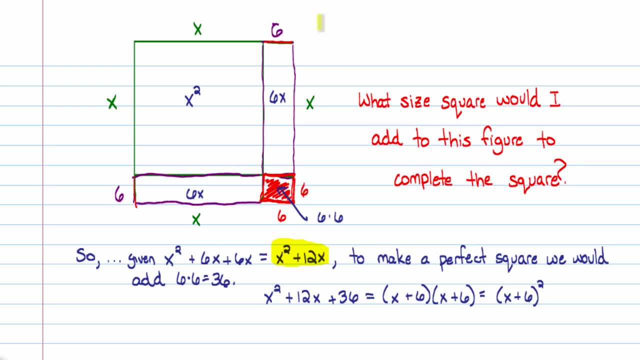 Now the question is: how do we get that 36?? What if I don't want to draw a picture every single time? Well, there's something to note about how we got that 36.. We got it because we said: well, let's take this 12x and split it in halves, right? 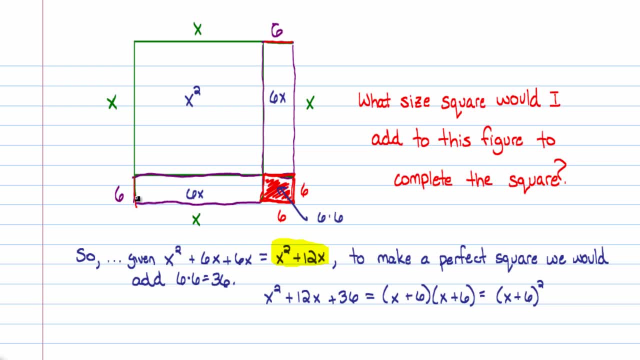 We had 12x here and we gave 6 of it here in this bottom block and the other 6x of it in the top block, And so we split that into two chunks. And what that did is it gave us a great idea. 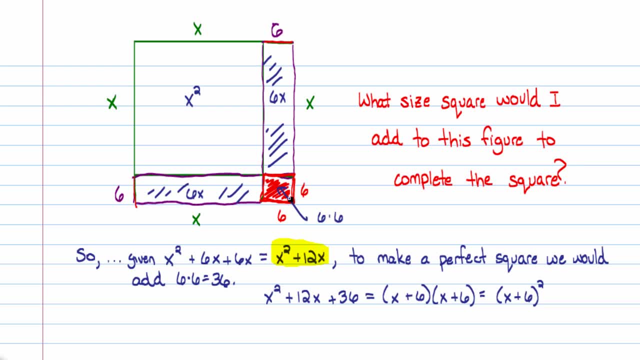 of what kind of square I want. I want a 6 by 6 square, Or in other words, I want a square that's half of that on each side. right, I want it to be half of 12, which is 6 on one side and 6 on the other side. 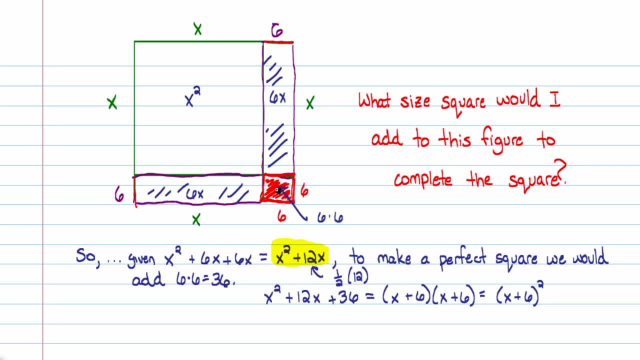 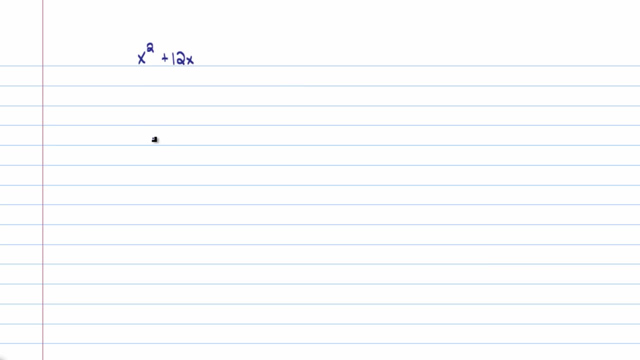 And of course we want to add that area in. so I have to multiply the 6 times 6, or in other words, that number squared. So let me write this down: We had x squared plus 12x and we are going to add: 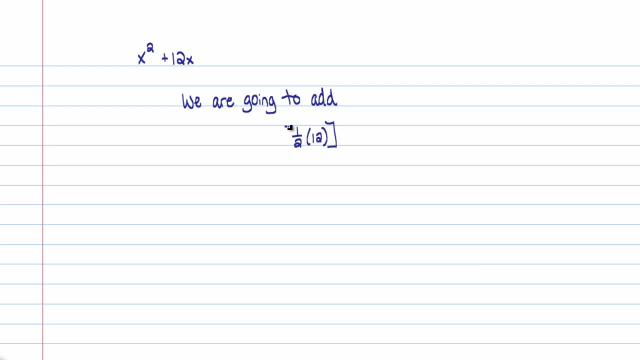 one half of that, 12 squared to make a perfect square, And if you think about that, that means x squared plus 12x, and then one half of 12 is 6, so we're going to add 6,, but being squared. 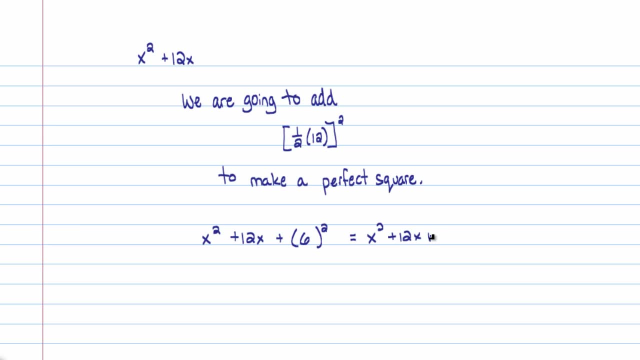 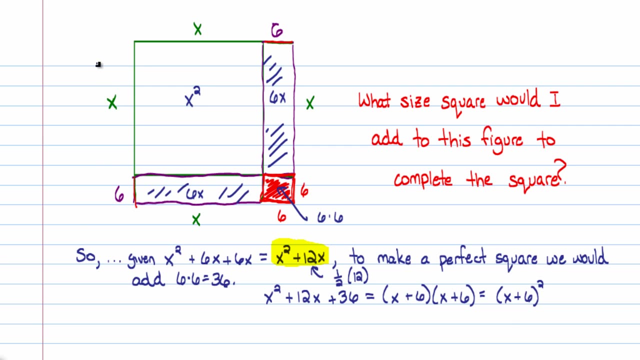 which is x squared plus 12x, And that was that polynomial that we were able to factor just a moment ago. Notice, by the way, the side length of this square is x plus 6 by x plus 6, which is exactly what our factorization turns into. 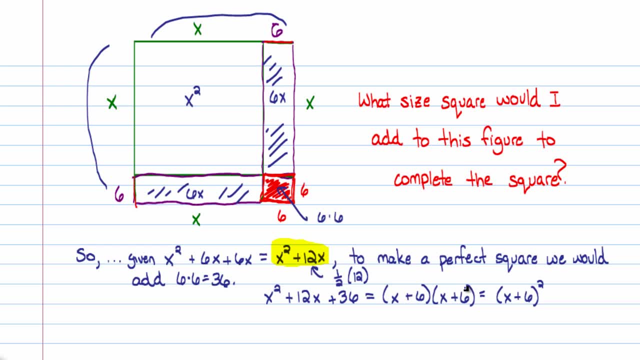 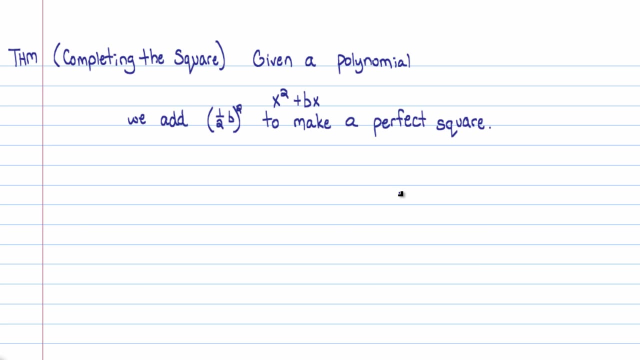 So let me write down the theorem for completing the square and then maybe we'll do a few examples of how to complete the square before we go into solving quadratics using this. Given a polynomial of the form x, squared plus some number times x, 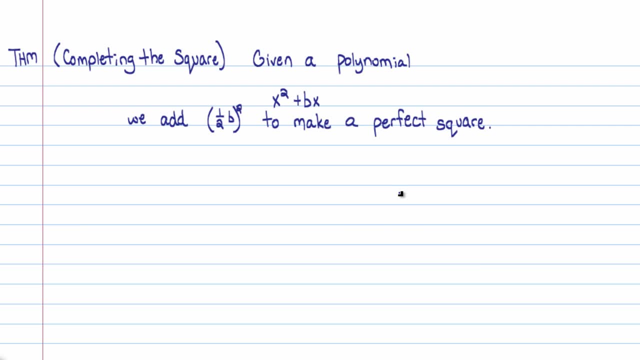 we just add half that number, in other words half b squared, to make a perfect square. That is how we complete the square. Now I want you to note a few things here. The coefficient on x squared here is just 1.. 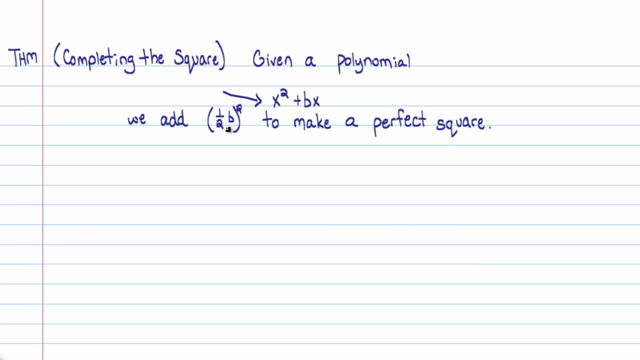 It's not a 5x squared plus bx. It's not a negative 2x squared plus bx, It is an x squared plus bx. It's very important. You cannot complete the square otherwise, Or if you try to, you have to make some type of adjustments. 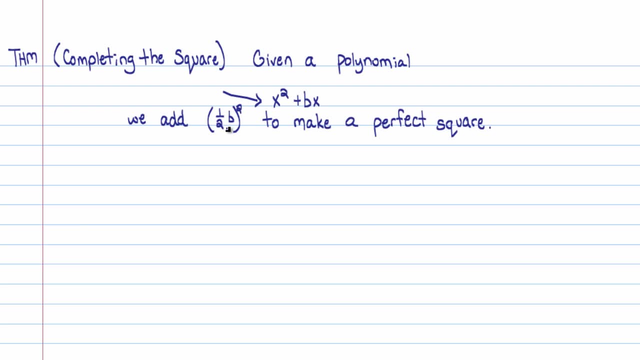 Another thing that I want you to know is if you're given a polynomial- this is saying that to complete, to make it a perfect square, basically you're going to have to change what that polynomial is. It's like if somebody gave you $5. 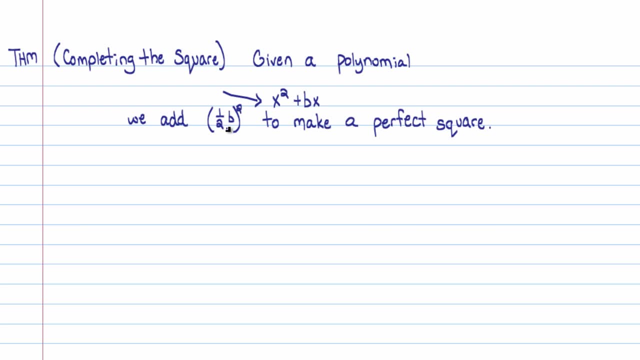 and you want to rewrite it. What I'm telling you right now is: rewrite it as 5 plus 1, or something like that. In other words, I'm making you change the polynomial, which seems pretty wrong, and it is pretty wrong. 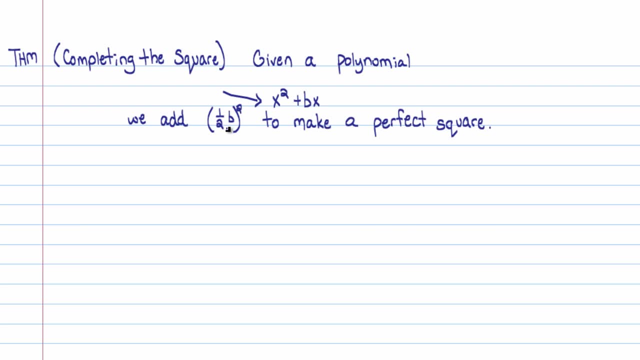 You shouldn't actually change the value of a polynomial. We'll talk about that in a moment. but we need to get used to the idea of actually being able to make a perfect square, given a polynomial. So we're going to work on that skill first. 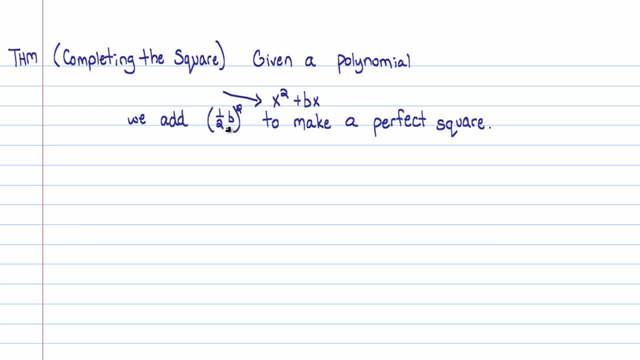 and then, after we're done working on that skill, we'll talk about: well, how do I readjust so that I'm not really changing this polynomial, I'm just changing the look of it. Another thing I want to mention is the reason why you learn completing the square. 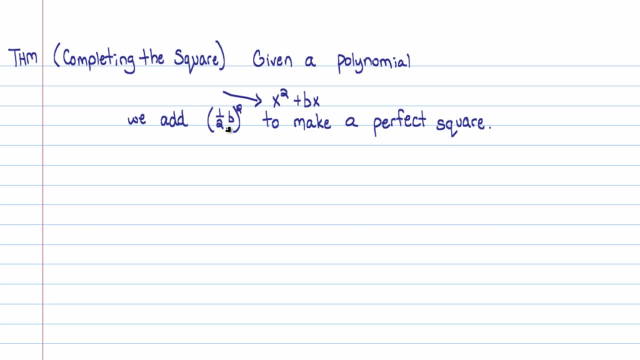 other than it being just kind of an interesting idea, is really, honestly, to prove a major theorem in mathematics called the quadratic formula, And that is the biggest reason why we learn completing the square. Now some instructors may force you to use completing the square. 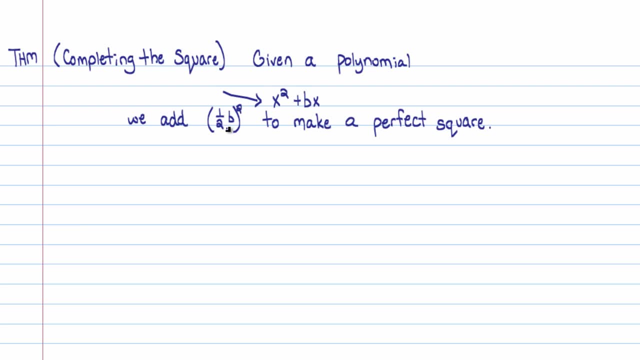 to solve problems in the future. If you're one of my students, I don't personally believe in that. I think that you should use every tool at your disposal to be able to solve any equation handed to you, so nobody's going to force you. 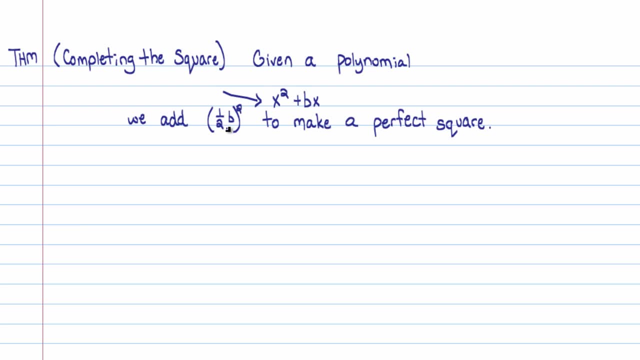 in the real world to solve something a specific way, And I don't believe that you should be forced here either, But you should have practice on making perfect squares. Now we're going to go through a series of problems and I'm going to give you 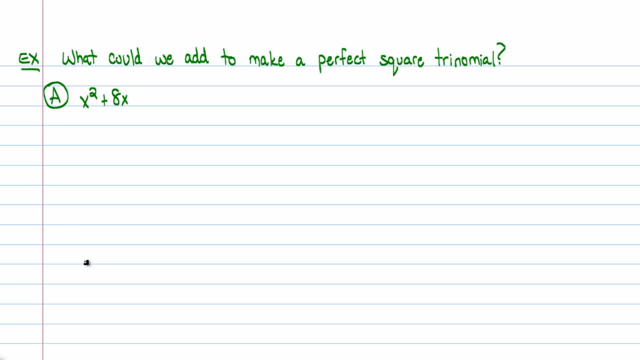 a few examples. They're all just going to be under this same heading. What can we add to make a perfect square trinomial? Each time I do an example, I'm going to speed up the process, But initially I want to make sure that 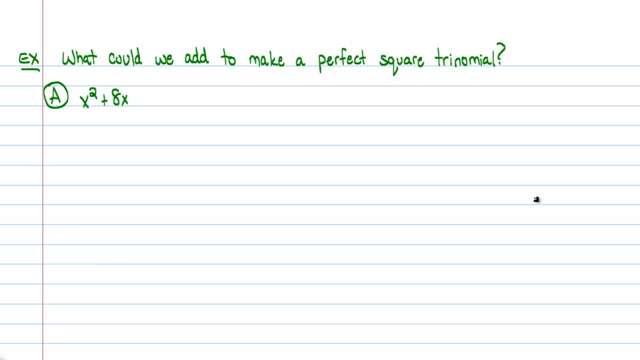 as you're watching this, you completely understand what's going on And also really understand the physical aspect of this. What this is saying is that you have some square that's x by x. That's what that first coefficient or that first term is saying. 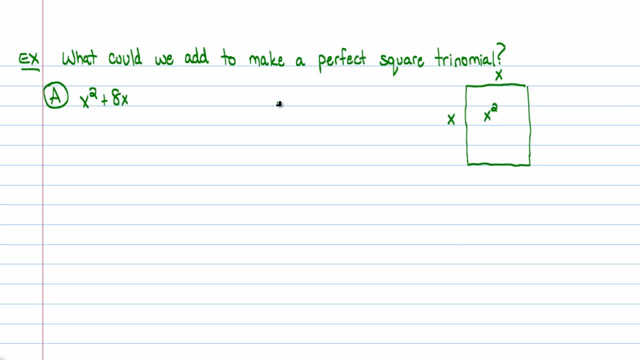 that you have an x squared term And then the next number there, that plus eight x means you have little rectangles hanging off the edge here on either of these, And this one has a height of x. This one has a width of x. 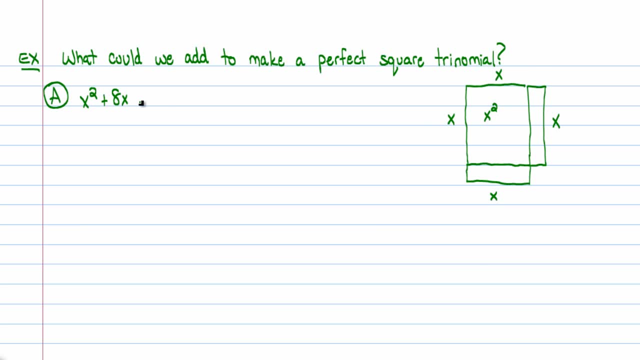 And the top one. I'm not going to write eight here. I'm going to split that eight into two pieces, A four and a four. So if you look at this, the area of that lower rectangle is four x. The area of the side rectangle is four x. 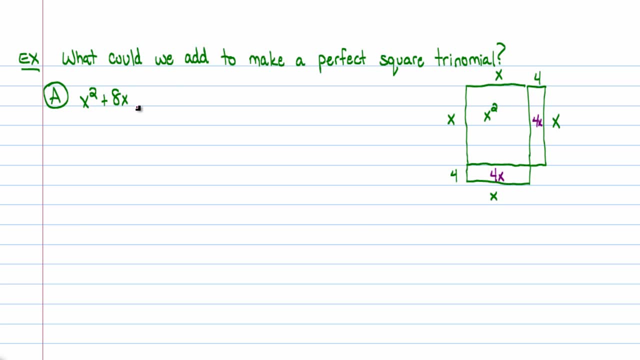 So we have x squared plus four x plus four x, Which is exactly x squared plus eight x, And what we're asking is to make this a perfect square, polynomial or trinomial. I just have to find out what size square I'm going to put in there. 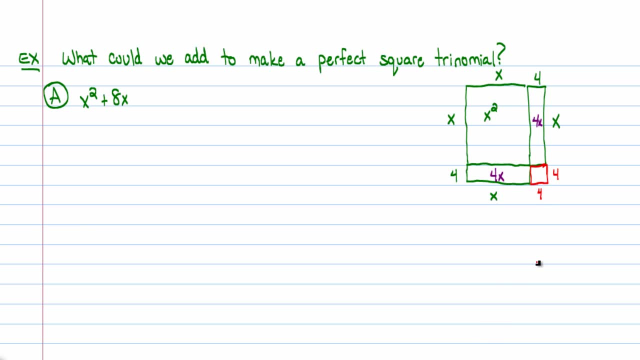 What size little piece? Well, I can easily see it's going to be a four by four, Which is a sixteen. That's the area of that. So, really, I'm going to add sixteen. That's the geometric interpretation of it. Is that you're going to add sixteen? 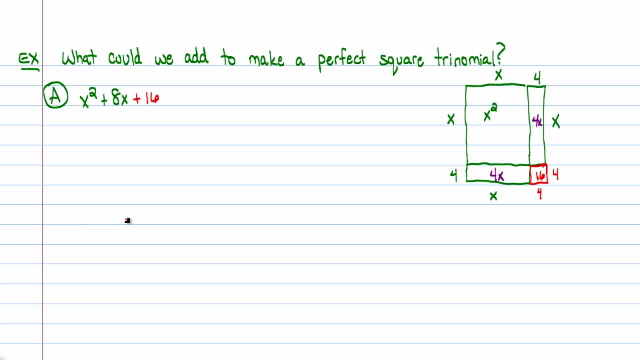 Now, often students want to just rush through this headlong and just memorize something. that works really well. But I'm telling you, if you know how to do this- this picture- then that will lend itself to a better understanding of completing the square. 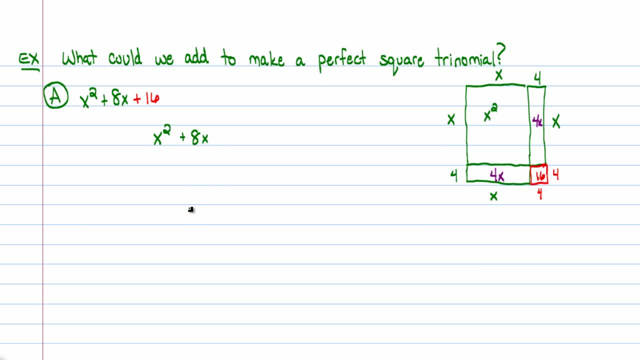 Completing the square. how we wrote it a moment ago as far as the theorem was, we would add one half of this number eight And then we would square it, Half of that middle term and square it. And if you look at that, 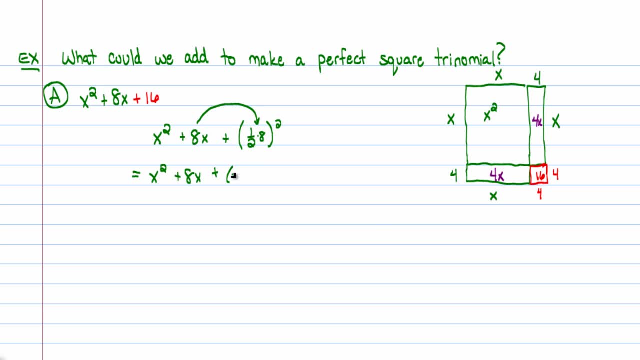 that's x squared plus eight. x plus half of eight is four Being squared, And that would be x squared plus eight, x plus sixteen. That's what we would add. We would add sixteen And, of course, to see that, to make sure that it's actually. 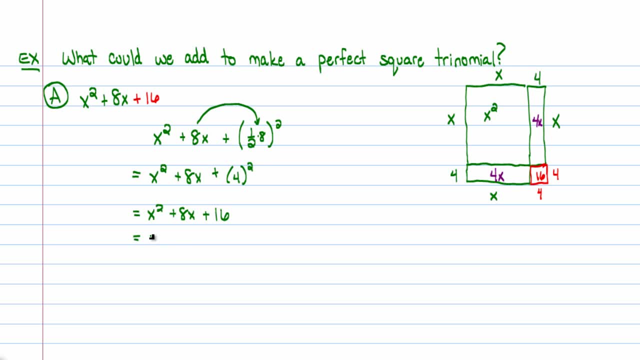 a perfect square. you can go ahead and factor this to check your work. Does this factor? Yes, it does. It factors to x plus four times x plus four, Or in other words, an x plus four being squared, Something I want you to note here. 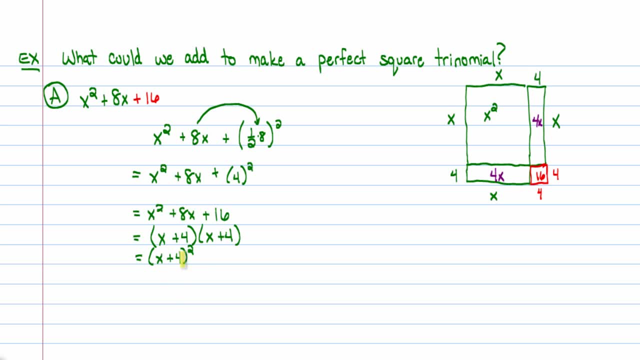 is that it factors to x plus four quantity squared. Notice that what we really added was a four squared, So I will show this every single time that we go through that when we add a number. so we started with x squared plus eight x. 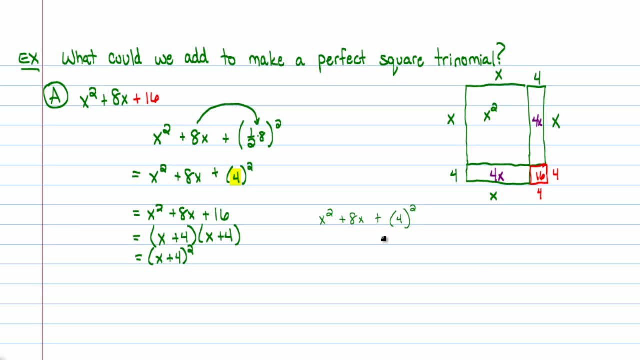 I will say: okay, add half of that eight, which is a four squared, And it will factor to an x. I'm just going to steal this x here and plus I'm going to steal this four squared. That's how it will actually factor. 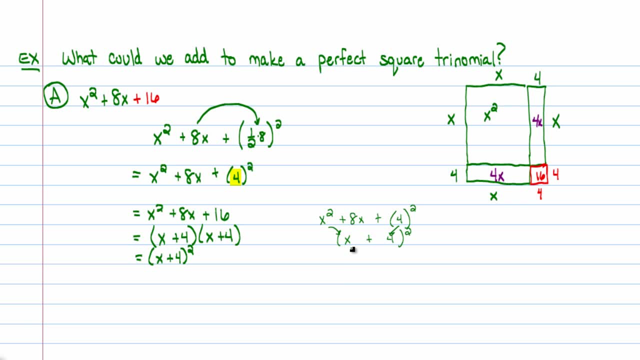 That idea of a quick factorization like that only works with perfect squares and is very useful for difficult factorings, specifically ones that involve fractions. So I will continue to do this in each of these examples. Again, let's see what we have to add. 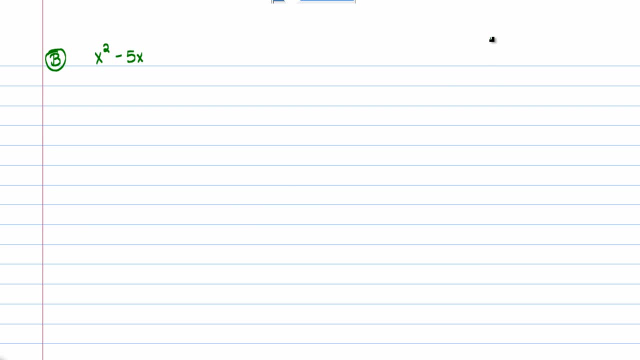 to x squared minus five x to make it a perfect square. Again, we are talking about an object x squared, which is represented as a square of length x on both sides, So that center, the area of it, is actually an x squared. 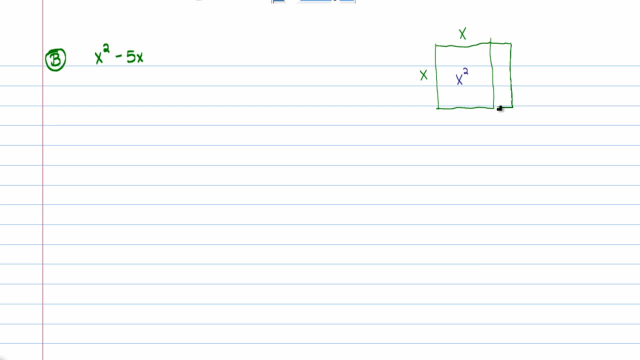 And then we have two little rectangles hanging off each side. This rectangle is of length x, or height x, I guess you would say. and this rectangle down here is of length x. And I'm breaking up that five into two pieces. I'm going to break it up into 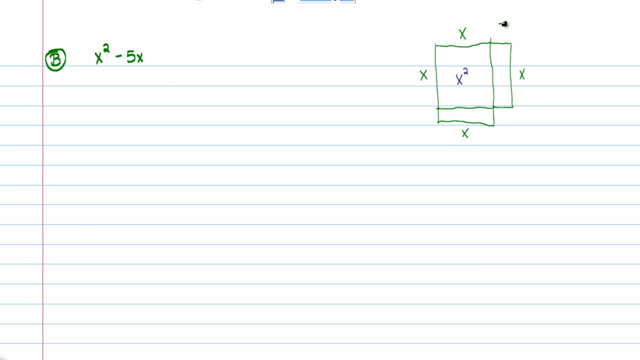 a five halves. in other words, I'm going to steal half of that five and put it here, and a five halves as well here Now, where the physical interpretation kind of falls apart with this. is that really, if I'm breaking up a negative five? 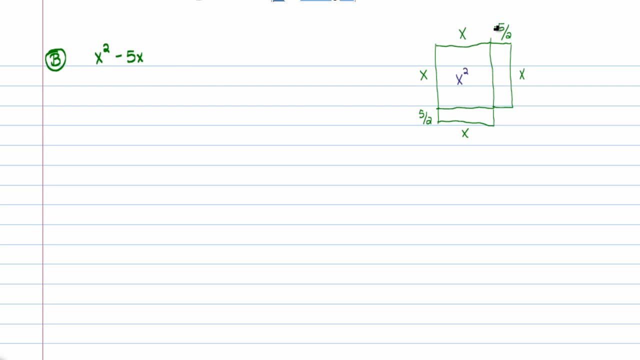 not a positive five. I'm breaking a negative five into two pieces, So it's actually negative five halves into negative five halves, Which is a weird interpretation, because the fact is lengths cannot be negative. but let's just pretend for now that we can still do this. 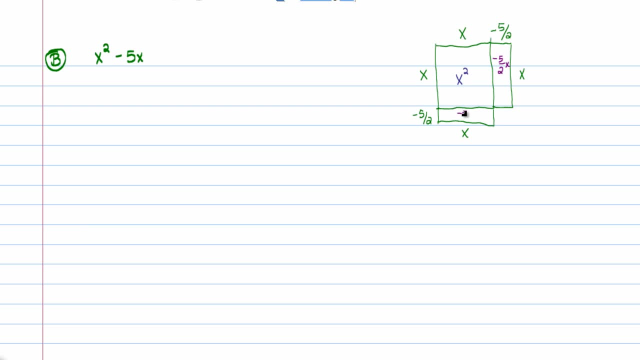 So this is going to be a negative five half x. This will be a negative five halves times x. And now I'm just going to ask: well, what size squared can I fit here? Well, it's a negative five halves by a negative five halves. 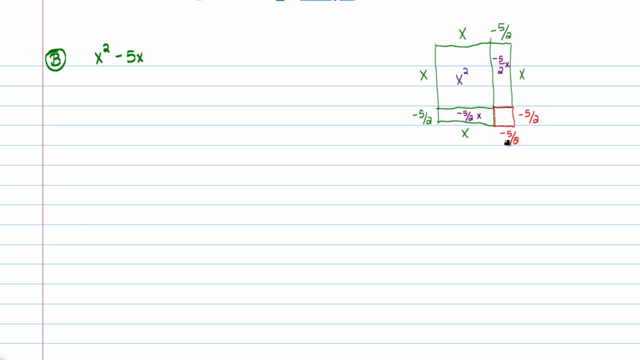 And, like I said, this is where the physical interpretation kind of breaks down, because lengths are not negative But the picture still works. I want to know the area of that chunk right there. Well, it's just going to be a negative. five halves squared. 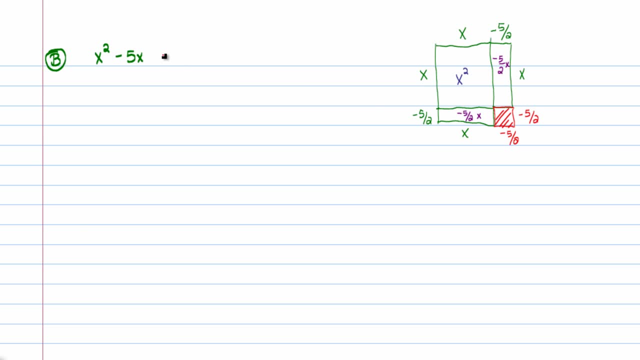 That's what I have to add to this to make this a perfect. square is a negative five halves squared, Which, if you think about it, is just half of this number. negative five, right, That's negative five over two. It's half of the number. negative five. 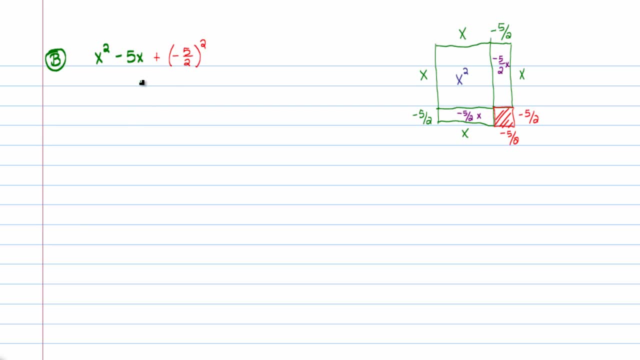 being squared. So really, if I want to write this as a perfect square now, it would be x squared minus five, x plus 25 fourths. Now, I told you a moment ago in the last example that what you really want to do when you're asked to complete the square 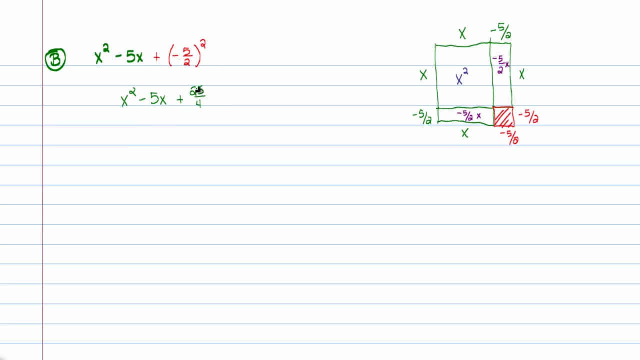 is you want to complete the square and then try to factor it if you can, And factoring this might be really difficult. If you look at this, two numbers that multiply to 25 fourths and add to a negative five, a lot of people might initially struggle with that. 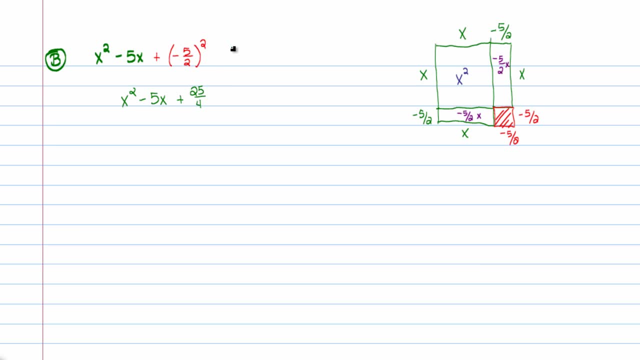 So I'm going to walk you through algebraically how I would do a problem like this. It's pretty straightforward but still very important for you to see. So we were given x squared minus five x and asked to complete the square. So what we did is we added: 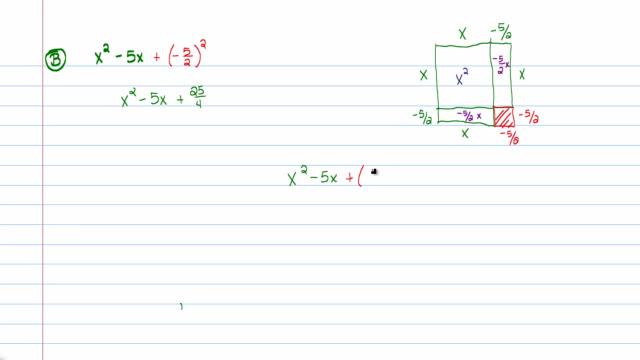 half of that negative five. That means basically a negative five over two squared. Now, just like I said last time, I'm going to steal one of those x's and one of these pictures in there, So this should factor to an x, because I'm stealing an x there. 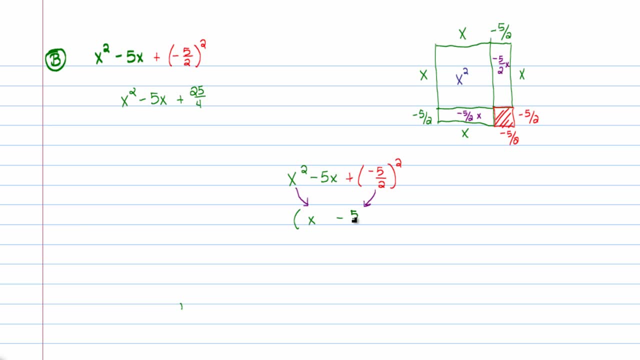 and this minus five halves quantity squared. That's how it should factor, because it should be a perfect square. So x minus five halves being squared. And if you look at the square that we wrote up here, its side length is actually x minus five halves. 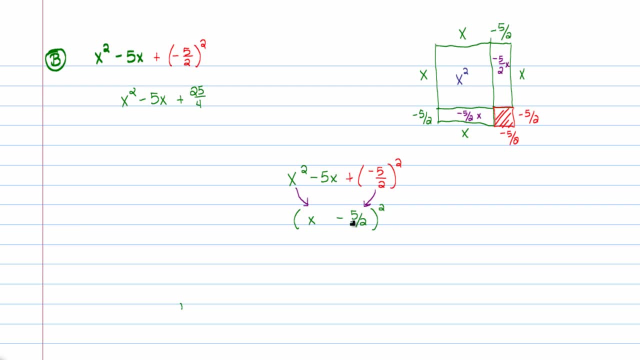 by x minus five halves, which is x minus five halves quantity squared. So we now will start going to a faster method. not method, really. We're not going to change anything. I'm just going to start speeding up Now in this example, 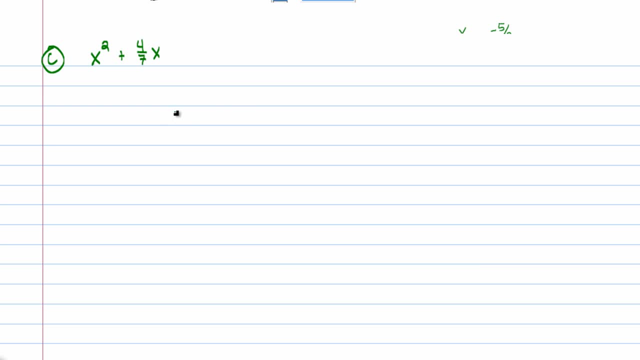 I'm not going to draw the picture anymore. I'm just going to immediately jump in and say, okay, I need to add something to x squared plus four sevenths x, so that I can complete the square. Now you should pause this video and try to do this yourself. 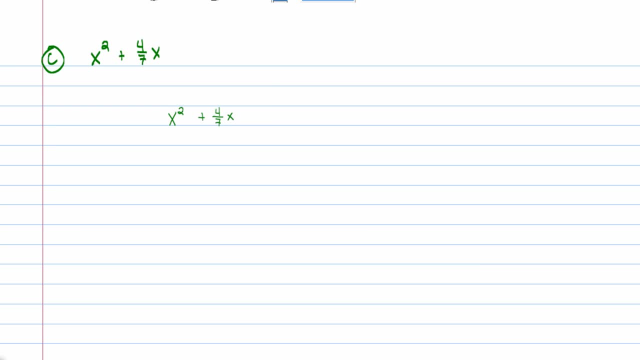 And then come back. hopefully you've just done that and see how I do it. So I'm just going to add to this half of that number, half of that four sevenths- and remember, half of a number means half times- and then square it. 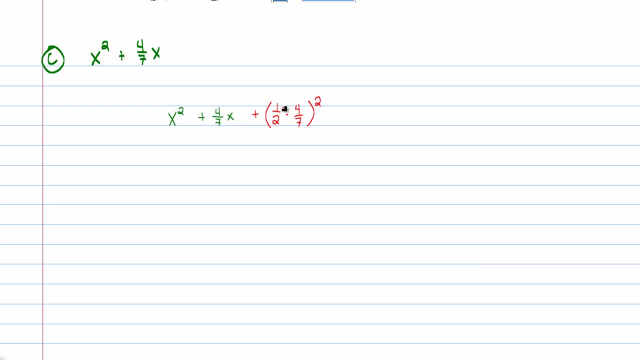 Of course it's a little bit faster to see that that means four, sevenths with a two times its denominator right. Half of a number means multiply that denominator by two, So this would actually be four over fourteen. but we can reduce that down. 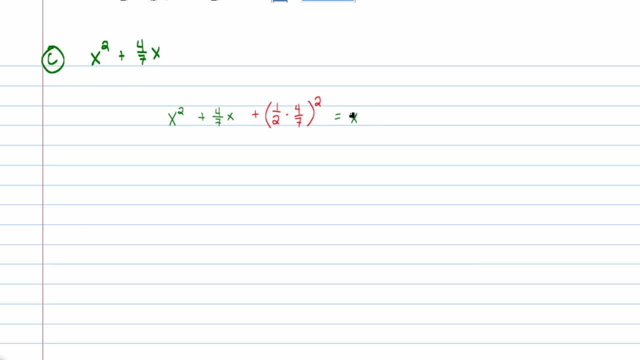 So let me just show you that This is x squared plus four sevenths, x plus two sevenths being square, And of course the number we're really adding here is four forty-ninths. So that's the number we're adding to this. 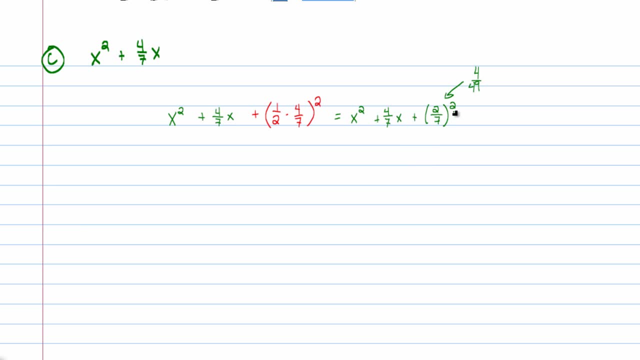 to be a completed square. However, I'm also going to probably say that you'll be asked to factor this result in the end, And it factors, just like I said a moment ago in the last two examples- actually steal that x and steal the inside of this. 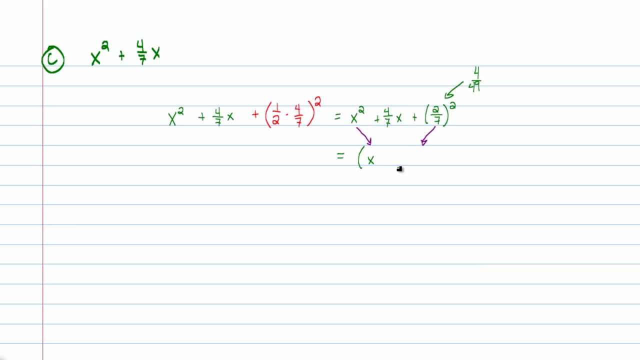 You'll get that this factors to x and that's a positive two sevenths being squared. So so, so important that you steal not only the four sevenths and steal half of it, but you're stealing half of positive four sevenths. 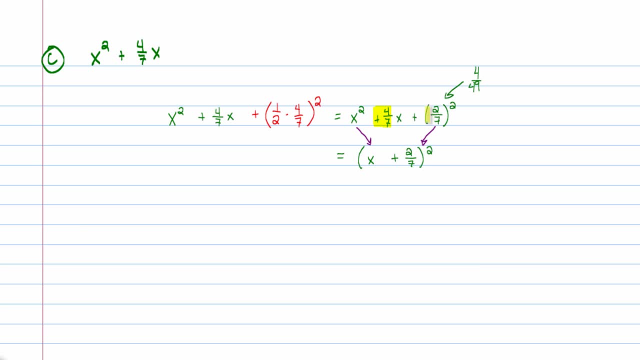 I know some people think: well, who cares if it was negative, because the square will get rid of it. so I'll never write a negative on the inside. But you should always write the negative on the inside, because it allows you to get this sign right here, correct? 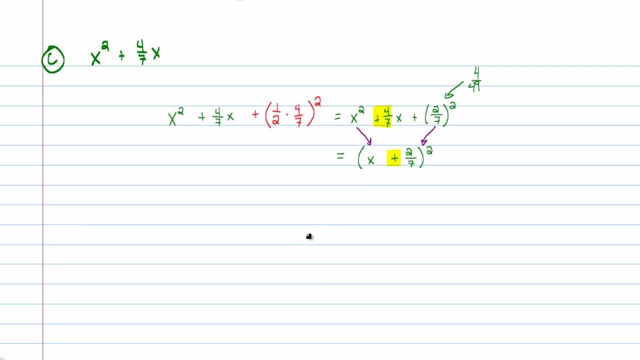 Just be very aware of that. Let's try another example. This will be our final example in this part of the lecture, And then after this, in the next part, we'll actually use this method to solve quadratic equations, which is kind of the area that we're talking about anyway. 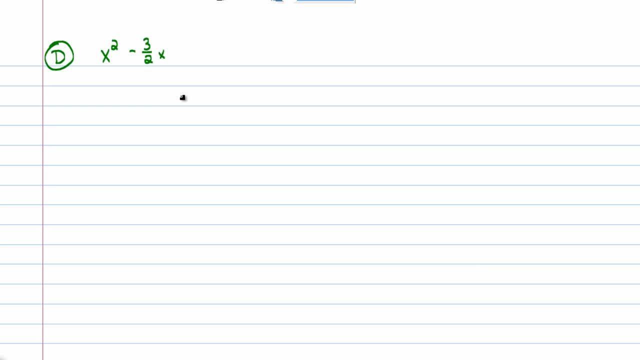 And in this example it's kind of like last example. actually I have an x squared minus a fraction times x, And what we want to do is add half of that fraction. So I'll write in the half times the fraction, which was a negative three halves. 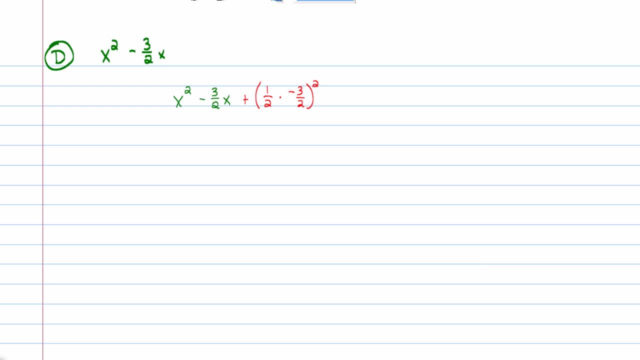 And then we'll square it And of course that can be rewritten nicely as x squared minus, three halves, x plus, and this would be a negative three fourths squared. Now, if you have an instructor that's asking you, what is this number?